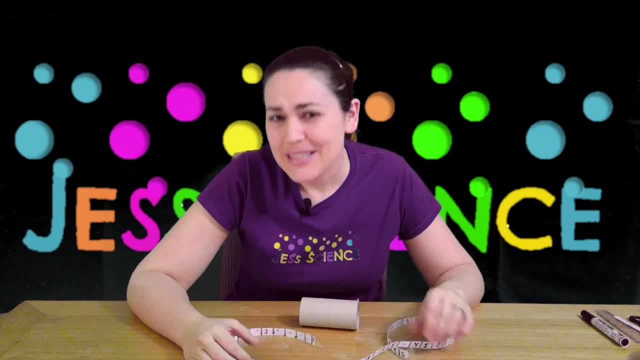 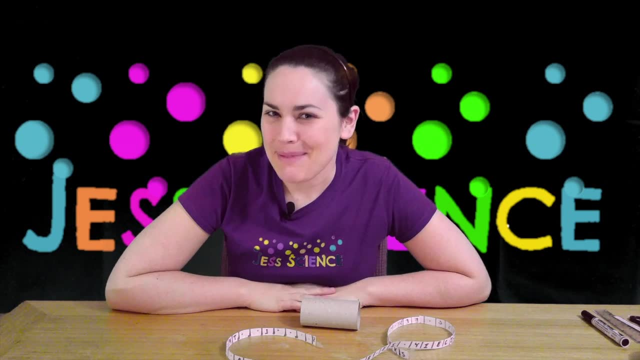 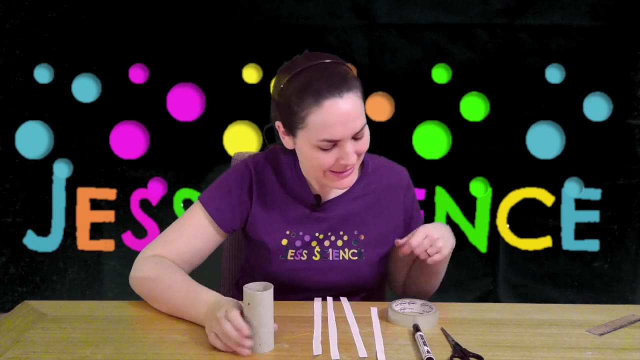 of being able to do a message that would be very difficult to read and lay out. And then you have the same size staff and you knew that's what you're looking for. Now let's find out what we need to make this To make your side tail cipher, you're going to need a toilet roll holder- some. 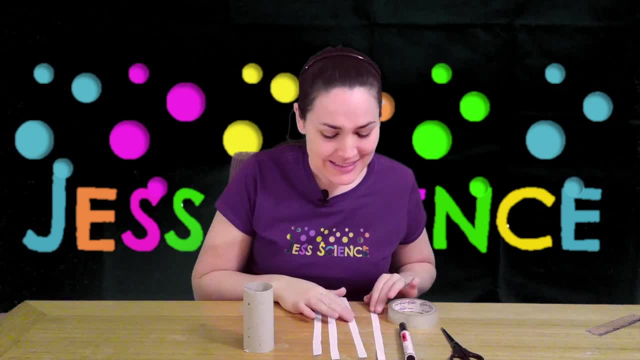 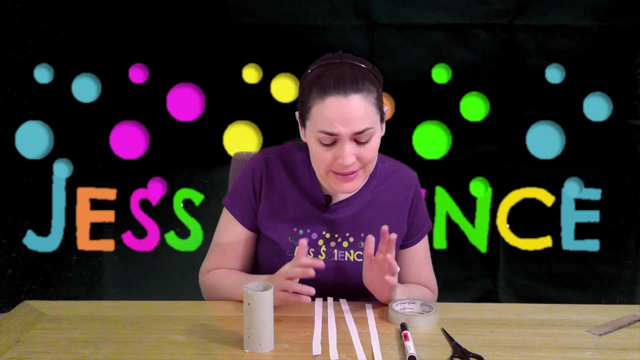 tape, a marker or a pen and some scissors. Now I've already pre-cut the paper, but you also need one piece of paper. I used an A4 or eight and a half by eleven. You can use a plain one or line one, whatever you have lying about, And I cut it into. 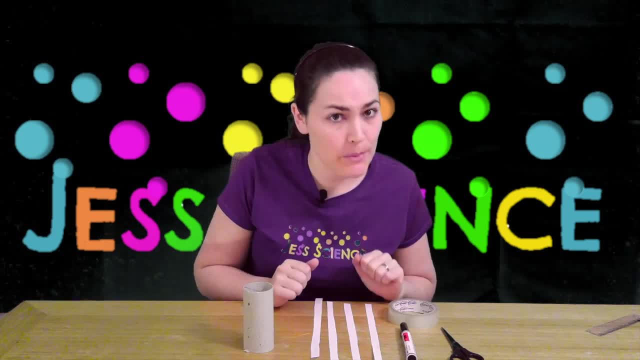 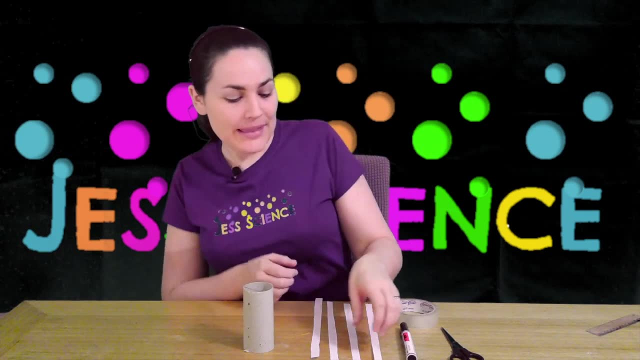 about one centimeter strips, and I did four strips of about one centimeters. So once I had my four strips cut, I have a little piece of tape on the ends of each of these. Now, what that means is I can tape them together. So if I just tape it, 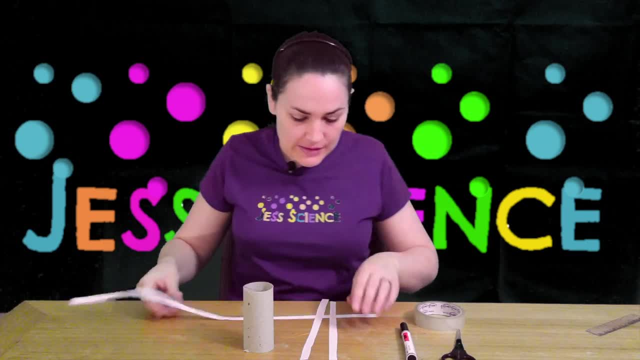 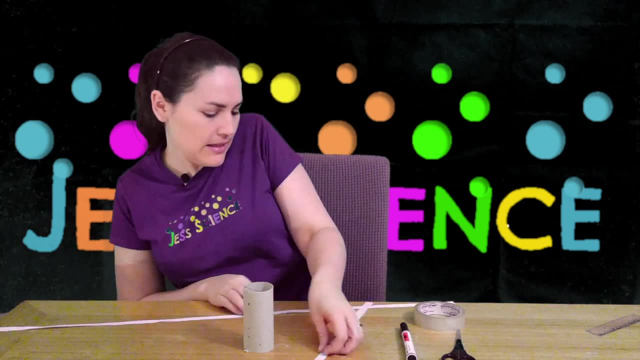 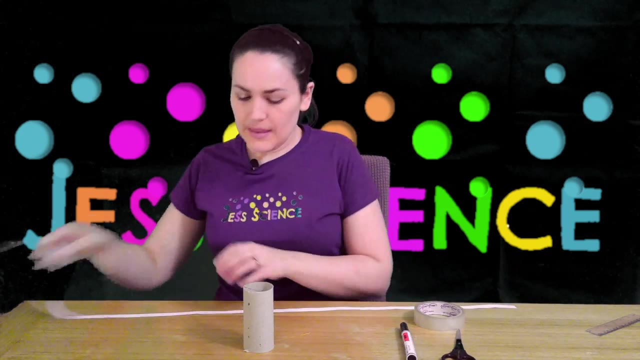 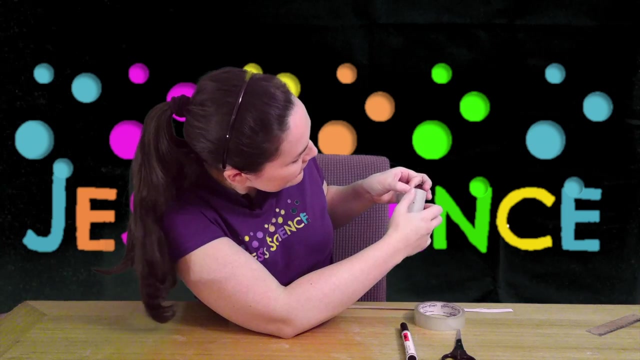 over here. I can line it up so that I've got four strips all together to make one very long piece of paper here. So if I just do that, there we go. Then I take my toilet roll holder and I carefully line it up at the very top and I gently wrap this around And if you want, you can. 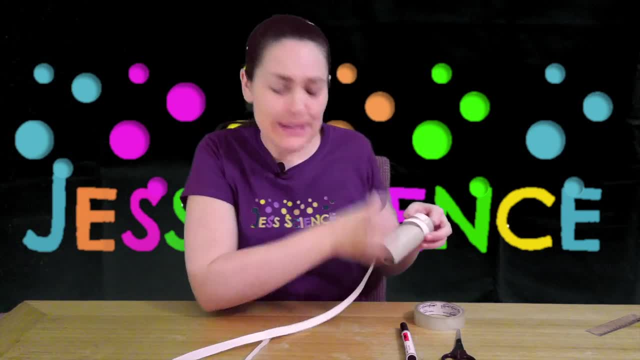 make your strip of paper a little bit wider too. It just means you'll have a little bit less space for your messages because you won't have as many lines going down. But wrap it around, and if you make it a nice and stud, it makes it easier to be able to wrap it around. 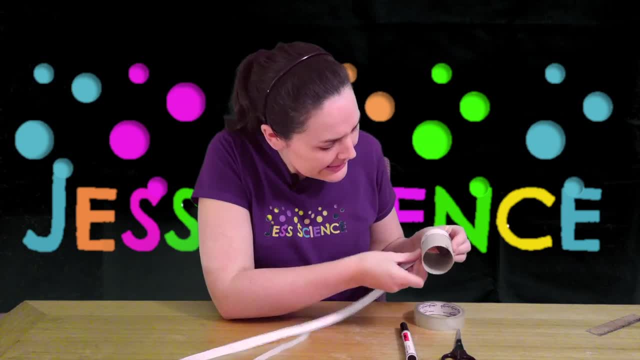 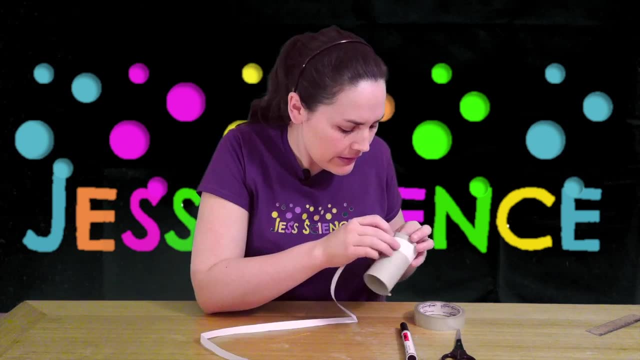 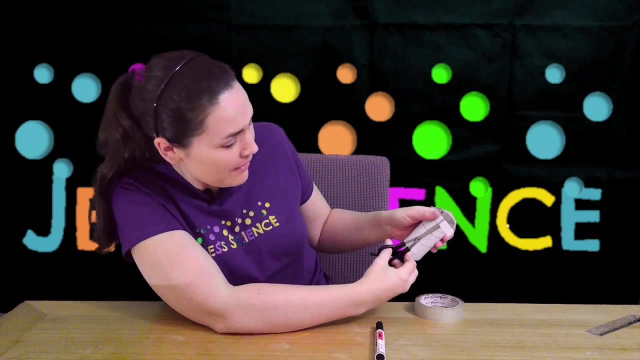 If you make it a nice and stud, it makes it easier to be able to wrap it around, wrap it to read it again later. All right, there we are. Then I can just cut the excess off, nice, and carefully Use a final piece of tape to tape it down here. 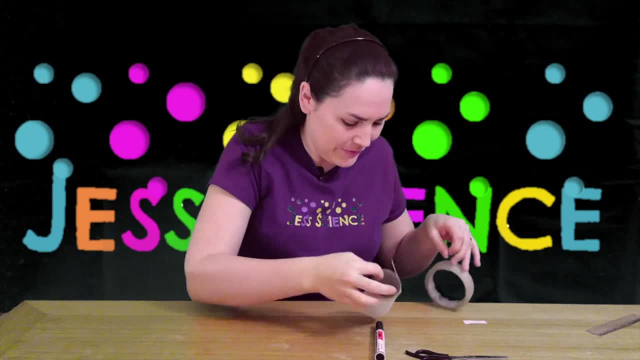 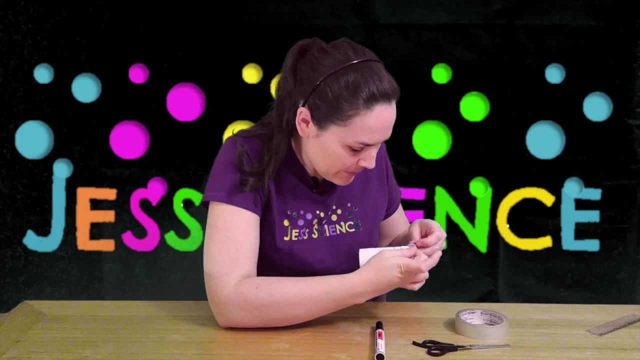 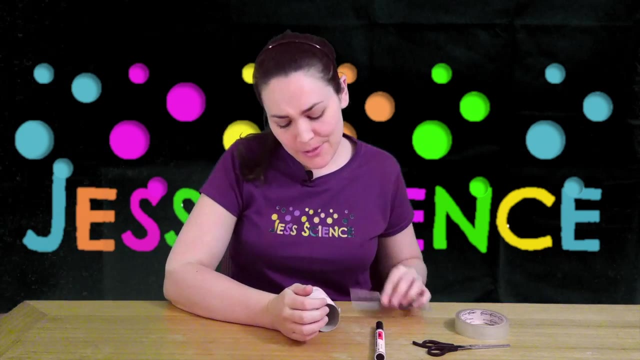 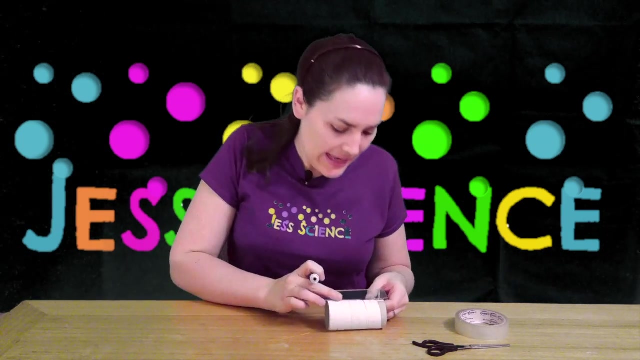 There we go: Carefully, cut the tape off and tape this one on: Wonderful. Now, if you have a ruler or an edge of another piece of paper, you can use that to make your lines. So figure out what your starting point is and draw out your lines across.